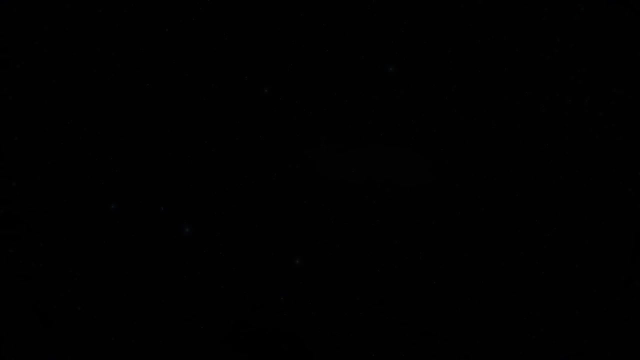 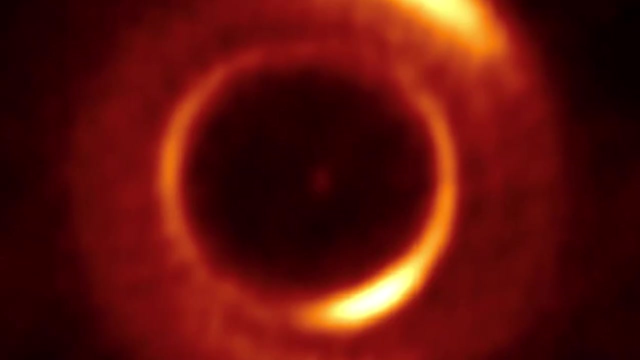 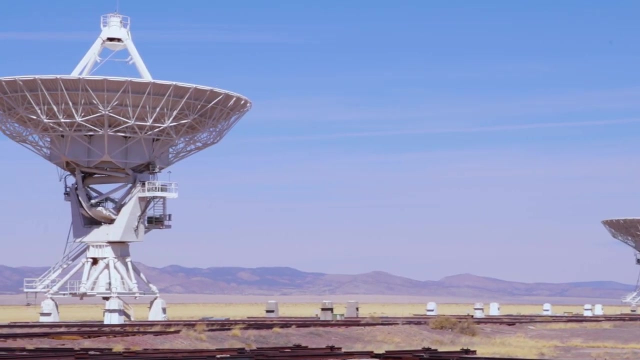 and nebulae, But there's also a lot you can't see, like jets from black holes and active regions of star formation in our own galaxy and disks of dust and gas that form planets. To see those you need a radio telescope. Most people are familiar with the optical. 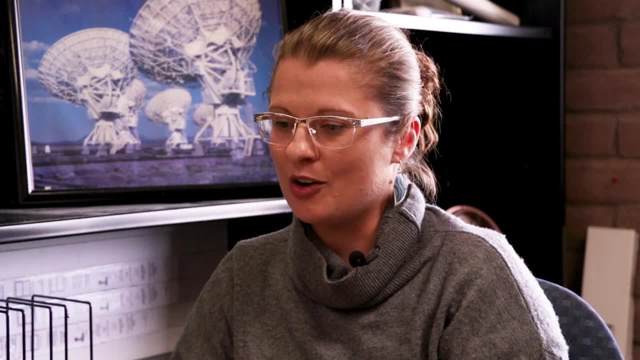 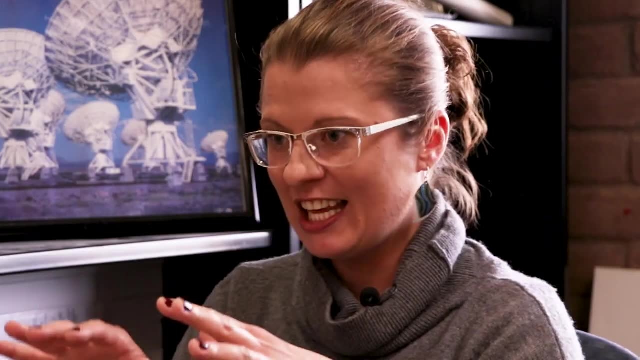 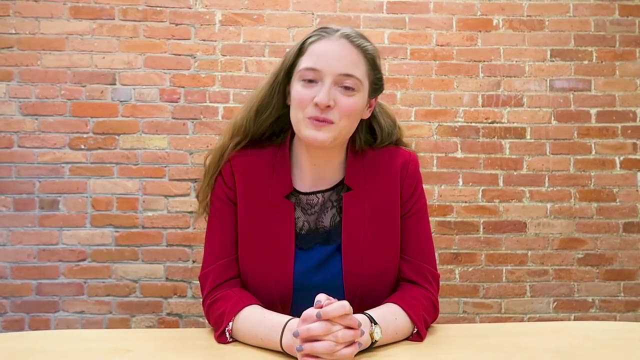 astronomy. obviously, because this is something that's part of the electromagnetic spectrum that our eyes are sensitive to. It's fundamentally the same type of radiation because it's electromagnetic radiation. Light comes in many different forms, with different wavelengths and frequencies. We can separate light into: 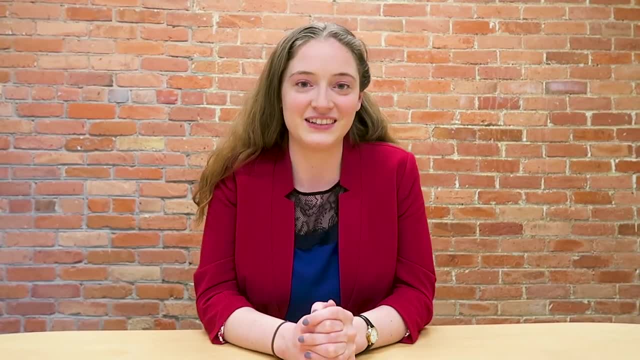 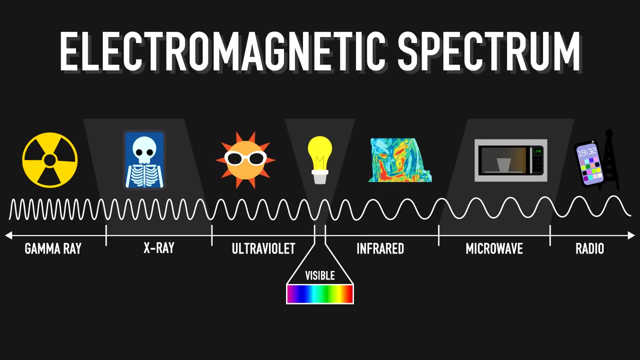 different categories based on the energy associated with light. For example, we have the light that we're sensitive to with our own eyes, That's optical light. We have lower energy waves, such as radio, and then we have really high energy waves like ultraviolet gamma rays. 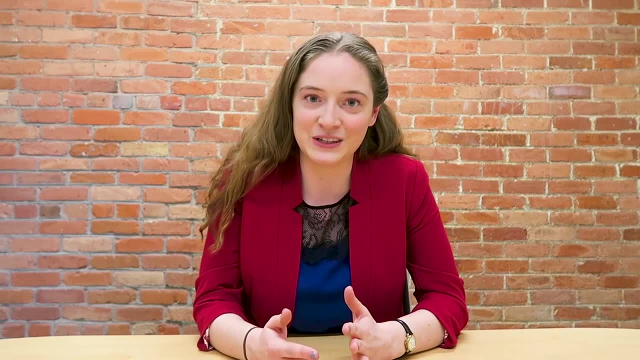 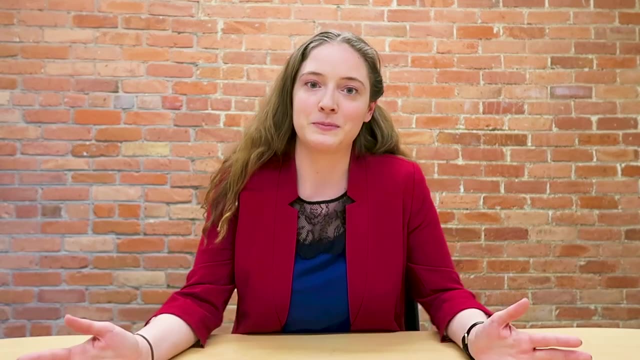 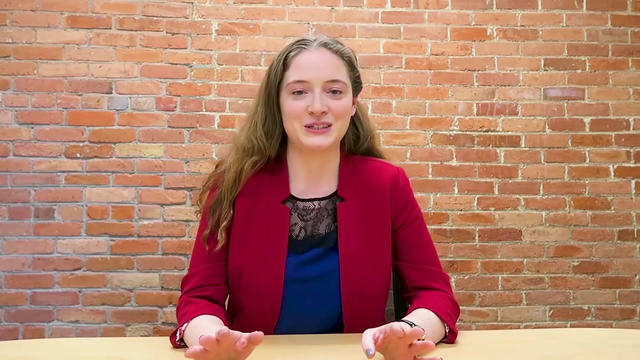 and cosmic rays. If we're only looking at the universe with optical light that we're used to, then we're only going to see a very small fraction of that full electromagnetic spectrum. We can still see stars, planets, galaxies, but we're missing a lot of other phenomena that we'd be totally blind to if we only 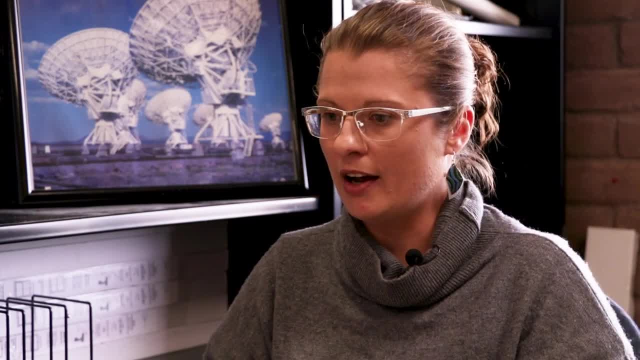 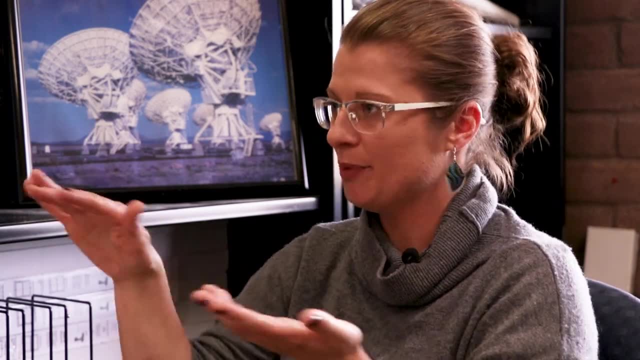 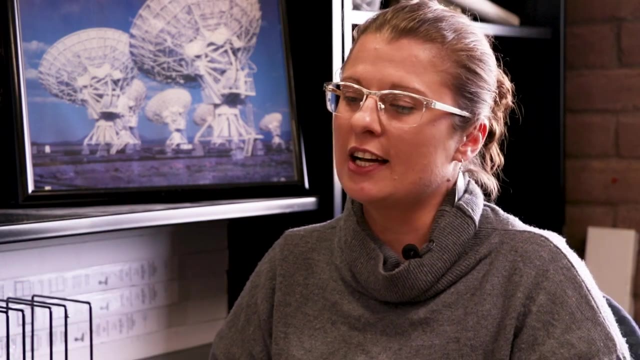 use the visible spectrum. Let's suppose that you have a galaxy and what you can see in an optical it will be the grand spiral, for example, or elliptical. You see the stars, you see the dust and so on. In radio, if that galaxy has a black hole, you will see the jets. 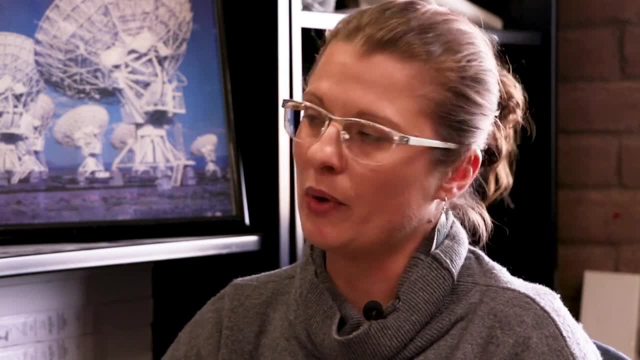 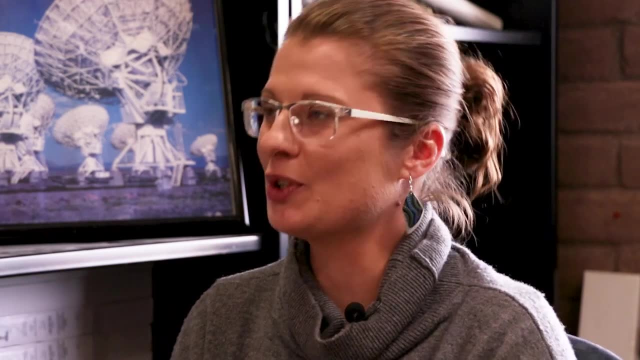 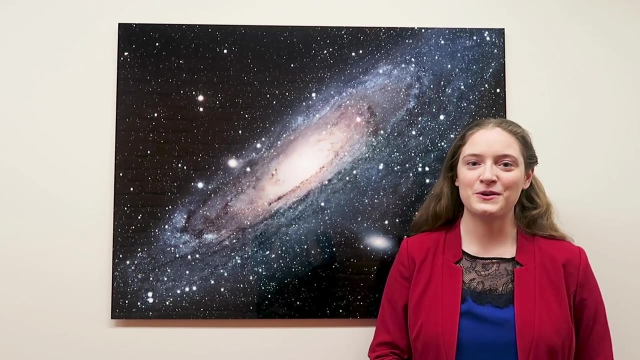 getting out Because we're looking at much longer wavelengths, the lower frequencies, the antennas are also different, So the way we detect the radio waves are slightly different than the optical ones. Observing in the radio is very important for the search and discovery. 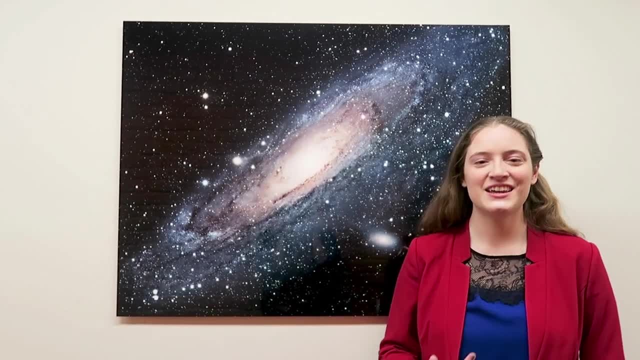 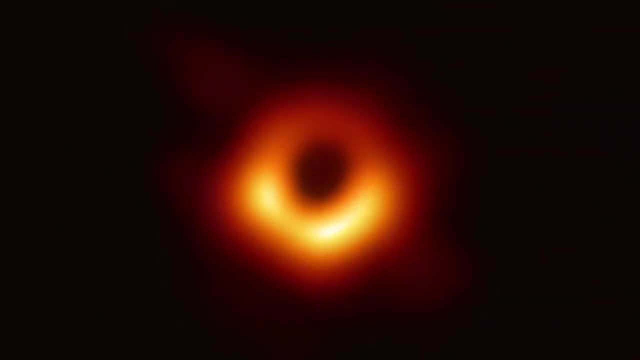 of supermassive black holes in the center of other galaxies. Recently, on April 10th, a team of astronomers publicly released the first image of a black hole in a another galaxy. To create that image, they had to use something called radio interferometry. 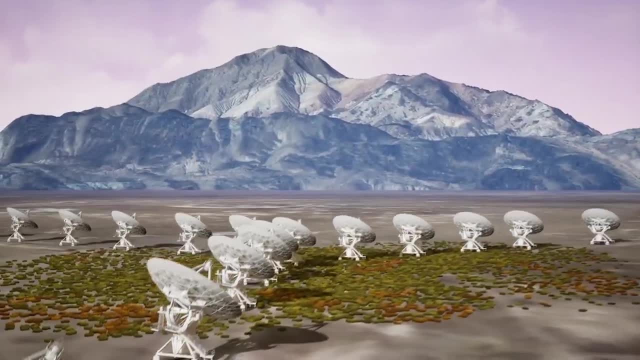 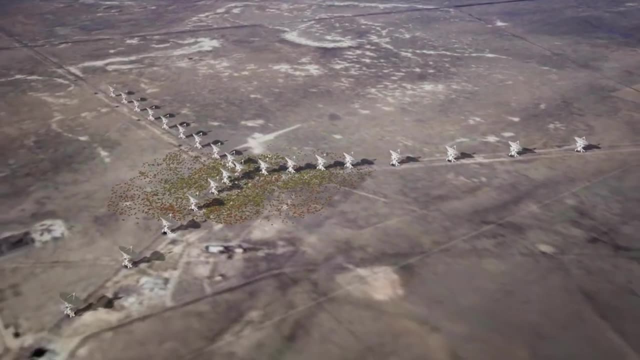 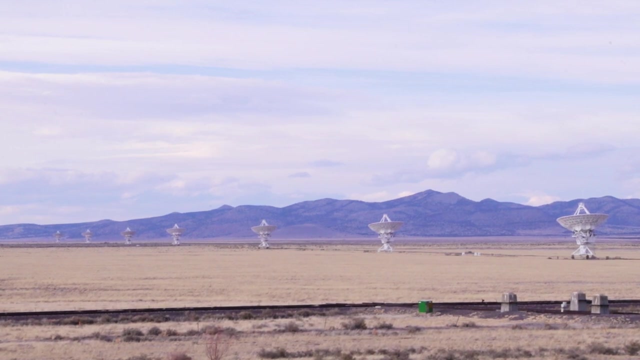 One of the most famous radio interferometers. out there is the Carl G Jansky Very Large Array. The 27 dishes on the VLA work together to combine a signal that simulate one giant telescope. So the VLA is able to achieve really high angular resolution. That means it can see very 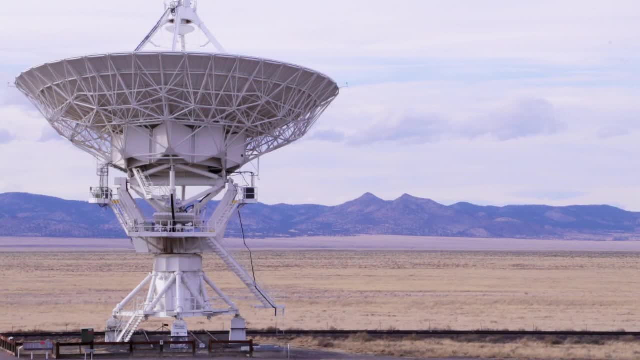 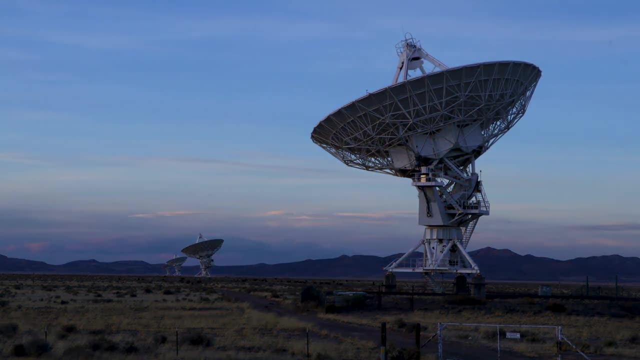 very tiny things on our night sky, For example a black hole. that's very, very, very, very, very far. Radio astronomy can also be done at any time, both day and night. That's because the sun is not a very 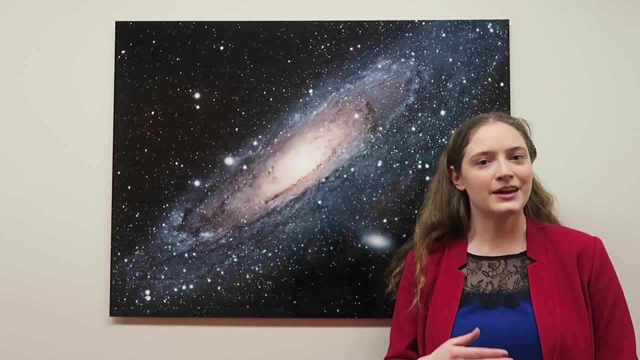 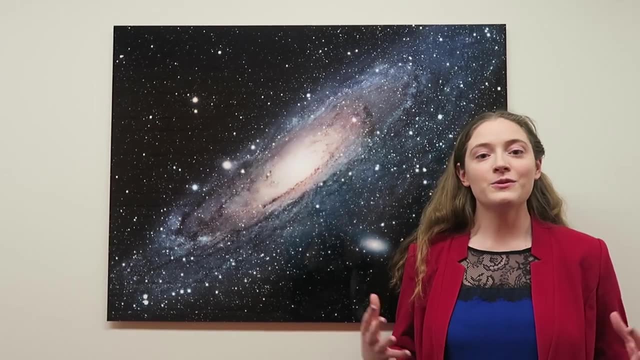 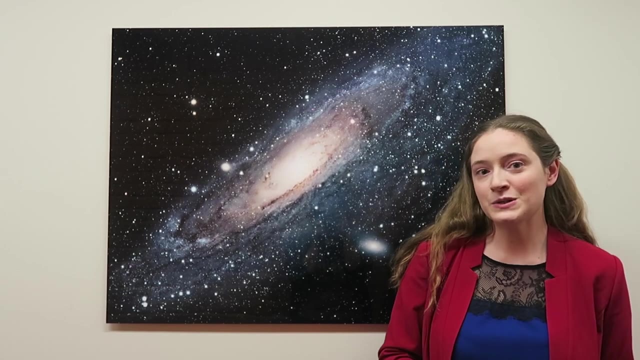 strong radio source. There are other radio sources that we need to be careful of, though, such as our phones, Wi-Fi routers, the TV, our car radio. These all work with radio wavelengths. Basically, anything we use to communicate with other people will emit in radio. If you're a radio astronomer, you want. 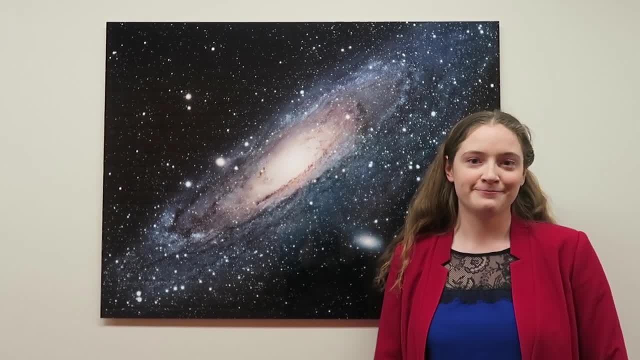 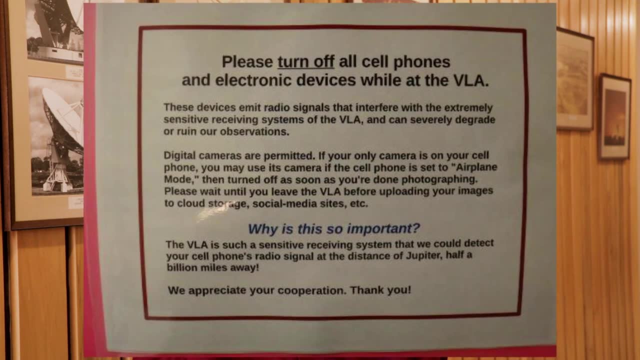 to build your radio telescopes far away from that sort of interference. When our tourists drive into the VLA they see signs saying turn off your cell phone, because your cell phone is in fact a very weak radio transmitter. That's part of the system. It's not supposed to hit. 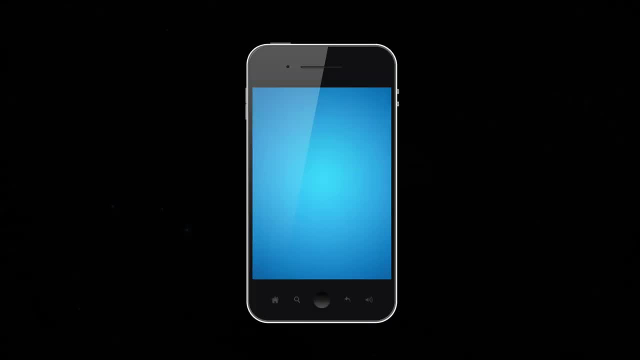 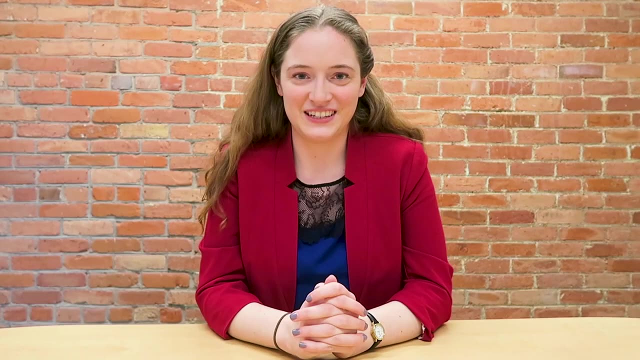 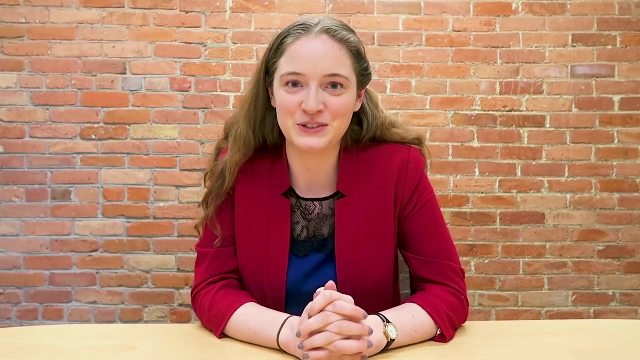 multiple towers, But if you had your cell phone, we could detect it if it were in orbit around the planet Jupiter. In order to mitigate this interference, there are a few frequencies that are off limits to the public. That includes the hydrogen line at 1420.4 megahertz and the channel 2 of your cell phone, which is at a volume of 500 MPa, Now the energy of the gas-fed radio 37 band, which ranges from 608 to 614 megahertz. There's even a large area of land in the United. 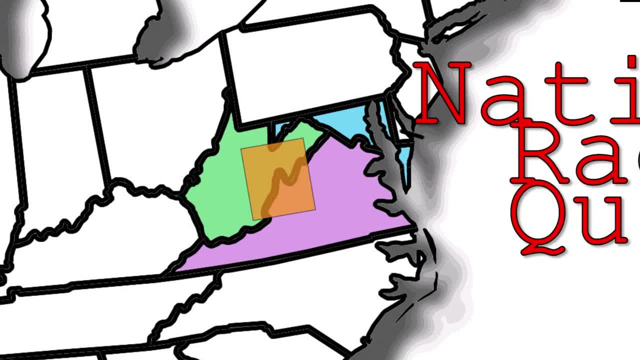 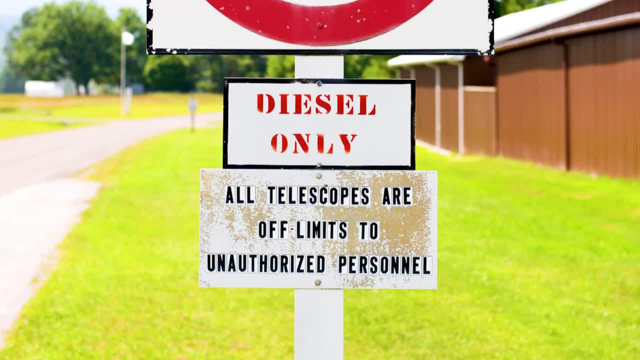 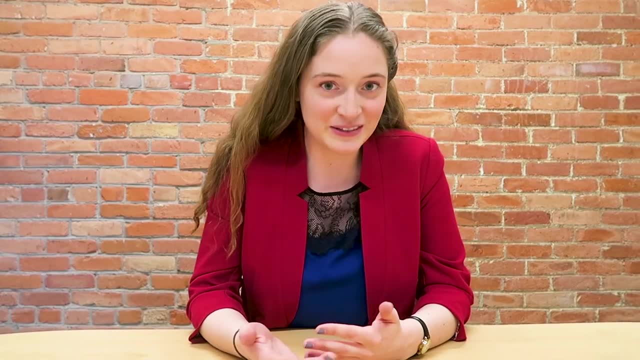 States. that's been designated as the National Radio Quiet Zone. It spans West Virginia, Virginia and a bit of Maryland and is home to the NRAO's Green Bank Observatory and the Sugar Grove Naval Radio Station. Emergency services and other broadcasters are allowed. some exceptions, but they have to coordinate with the Green Bank Telescope to prevent any sort of radio interference. If you're within 20 miles of the radio telescope itself and you use a microwave Wi-Fi router or even a phone call, it could have the observatory patrol knocking on. 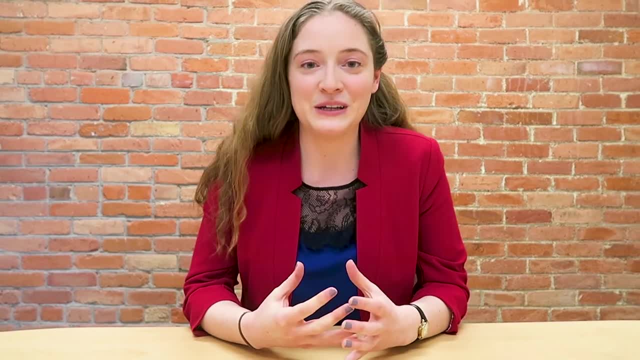 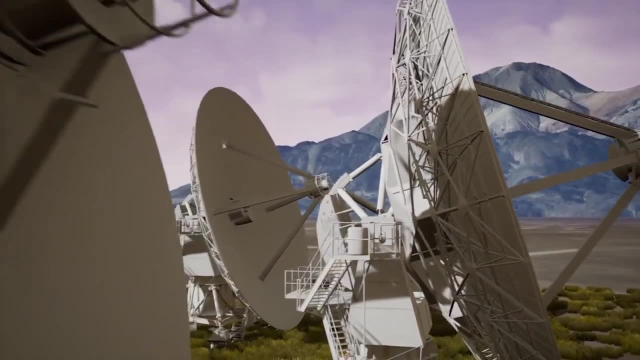 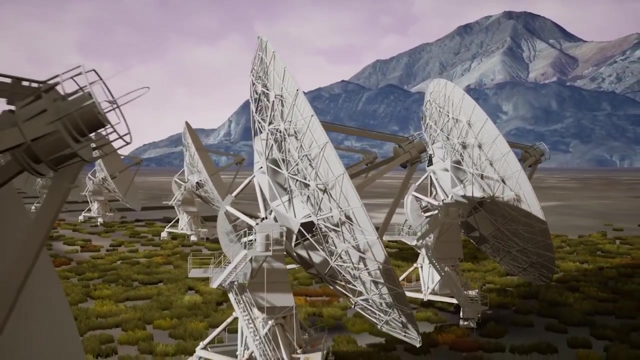 your door. These rules and regulations are in place to protect radio astronomy for now and into the future. Expanding our observing to lower wavelengths has already garnered some amazing discoveries in radio astronomy's almost century-long history, And the future is only going to bring more. 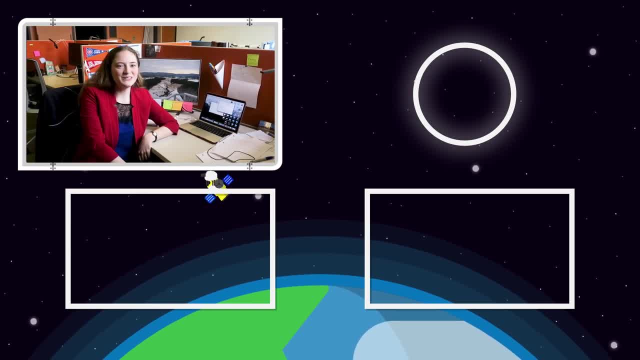 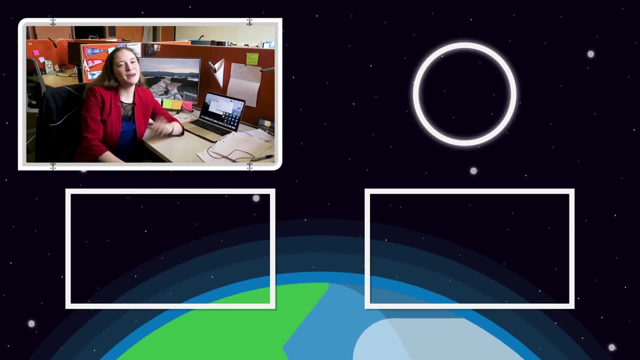 Hi everyone. it's Jenny. I was part of AGV for the past three or four years and I've since moved away from Tucson and I'm living in Michigan. now I'm a grad student here at the University of Michigan. I work with radio data every day. so if you have any questions about interparometry or 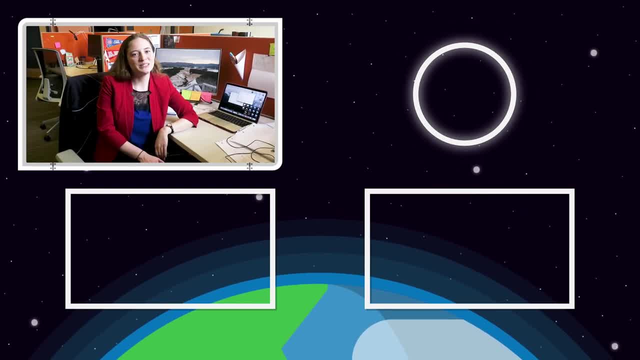 radio astronomy in general. I'd be glad to answer them, so just leave them in the comments And thank you for watching.